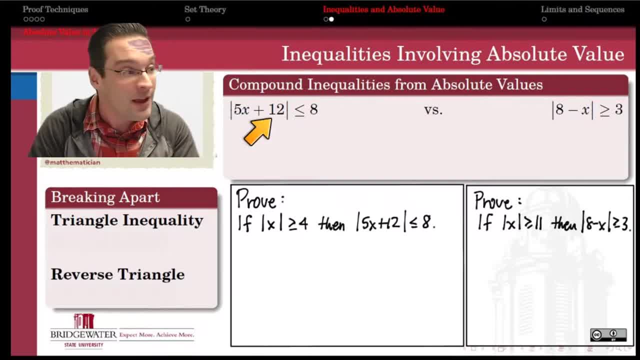 the left is saying that the distance between 5x and negative 12 is bounded from above by 8. So 5x is no more than 8 units away from the number negative 12.. So since my distance is being hemmed in, I'm. 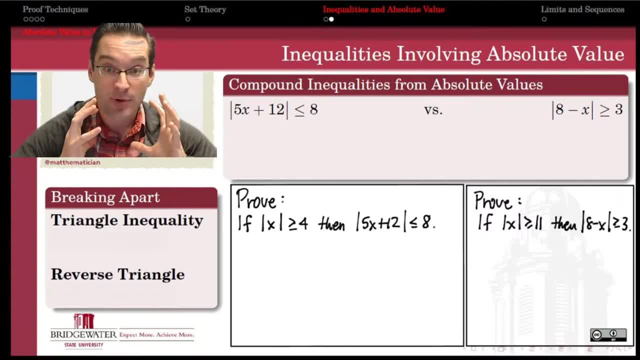 going to expect that my answer to this inequality is going to be a bounded interval, right? It's like we only give x a certain leash through which the dog can sort of run around, and it can't go any further away than that leash lets it go. That's what happens when an inequality with an absolute. 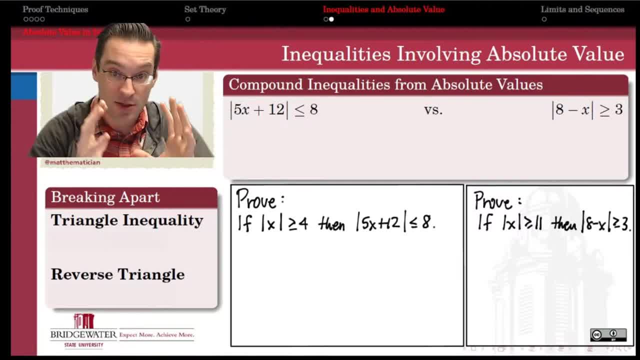 value is bounded from above. It constrains us such that our solution is probably going to be a bounded interval of the real numbers, Whereas in this example we're saying exactly the opposite. We're saying that x cannot get any closer to the number 8 than 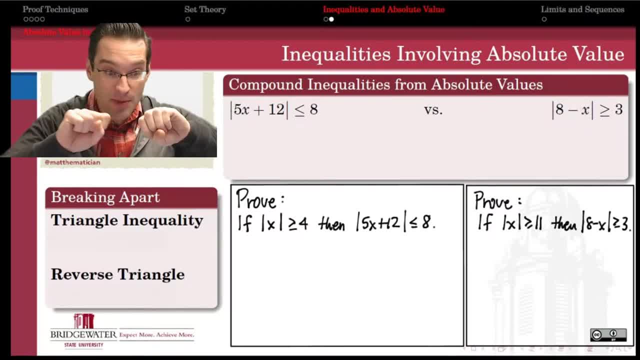 3 units, So x has to be at least 3 units away from 8.. So it's bounding x away from something rather than bounding it inward towards something. So what we expect is to have an unbounded pair of intervals, a union of an unbounded pair of intervals. that's going to be the solution set to this. 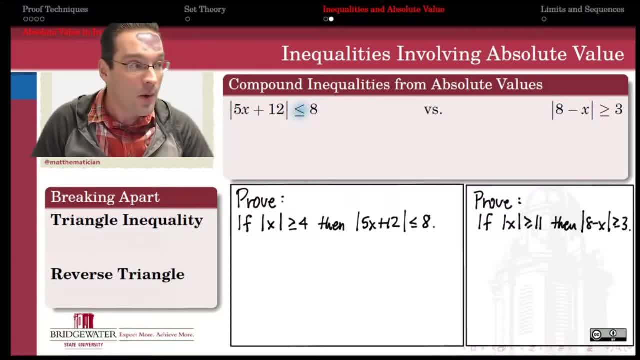 So what does this look like in the algebra when we actually solve it? Well, a less than or equal to is a graphing method where we say: if we choose a given four number, then to the infinity of x per 2 we go Caương into a scriptures for this equation, The simple calculator model approach. A lesser than or equal to a component inequality: less than or equal to. less than or equal to. This is usually the shorthand that we use for this. As we break it out into a compound inequality: less than or equal to. less than or equal to, We remove the absolutely values from the middle, 5x plus. 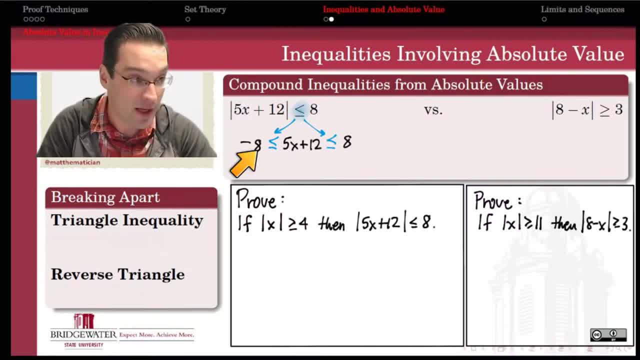 12. And we agree that this inequality is going to be satisfied whenever 5x plus 12 is itself less than or equal value from above. we can break it into one of these sort of three-part inequalities, and then we can just endeavor to solve this three-part. 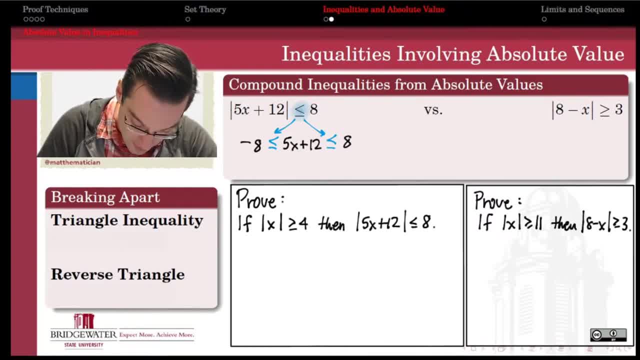 inequality using our usual set of solving and inequality steps, namely I would subtract 12 from all three pieces of this compound inequality and since f of X equals X minus 12, is an increasing function that's going to preserve the sense of all my inequalities. don't have to reverse my inequalities and then I'll. 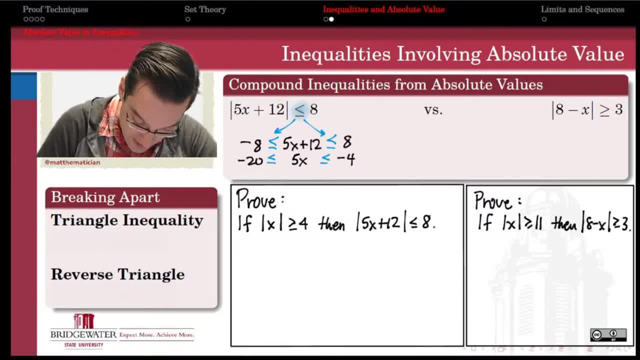 divide by 5, which, since f of X equals X over 5, is also an increasing function. I also keep my inequality symbols the same way. my X stands alone. I'm gonna get negative 4 fifths over here on the top and I'm gonna get negative 20 divided by. 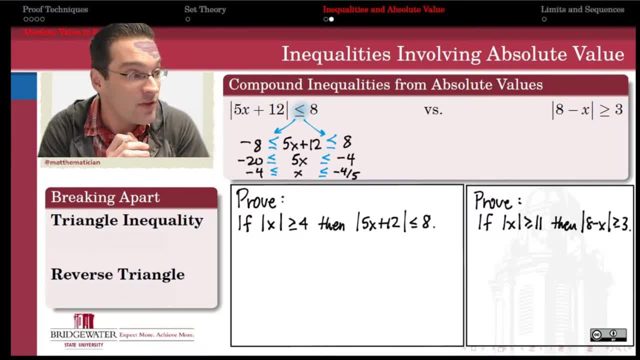 5, negative 4 down here on the bottom. so now we've solved this inequality. if we wanted to, we could write as a solution set that X must belong to the set negative 4 to negative 4. fifths, as an interval of the real numbers inclusive of both endpoints, I'm using 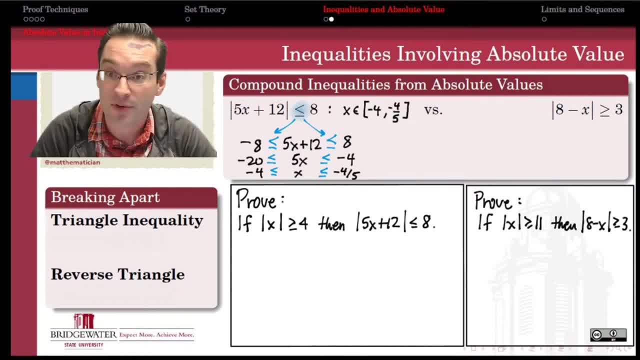 square brackets here, because both X equals negative 4 and X equals negative 4. fifths are a part of my solution set. so that's how to do it. when your inequality is bounded from above, when your inequality is bounded from below and we're trying to keep X at least 3 units away from 8, it's like. it's like a. 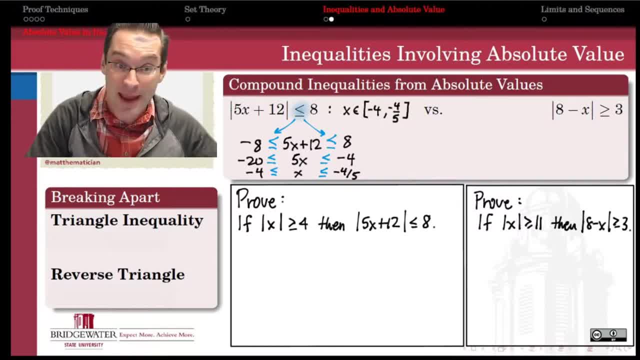 restraining order, in a way. right X cannot get any closer to 8 than 3 units, and so what happens here is that it breaks into again a pair of inequalities, but instead of those inequalities being joined together by the implicit logical, and that comes with this triple inequality, this time it gets connected by the logical or, and we have 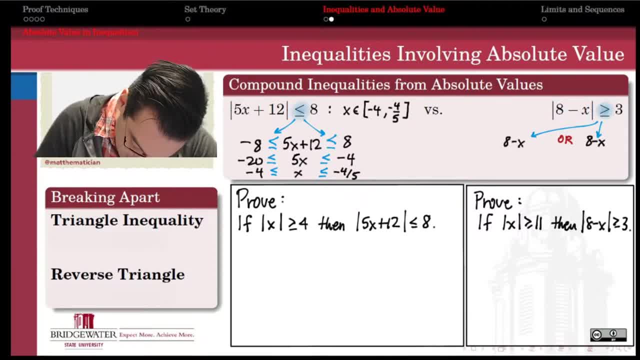 8 minus X, in both cases minus X. so this inequality will be satisfied if 8 minus X itself is greater than or equal to 3, but would also be satisfied if 8 minus X is less than or equal to 3 negative 3. so notice, in both cases, what ended up happening is we just took this. 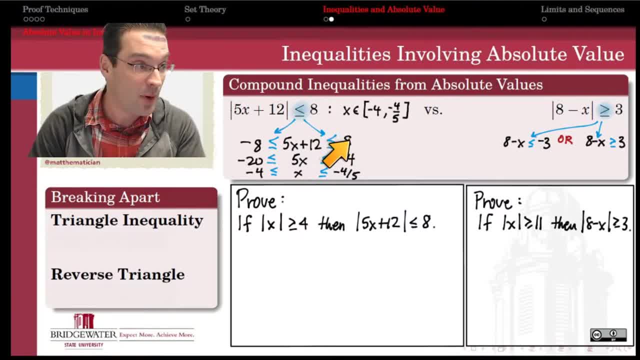 this constant that was on the other side, and we had both itself and its opposite as part of our inequality. and when we put in its opposite, the sense of its inequality symbol, just reversed right. and the only big difference between this example in this one is that we have an illogical, or here instead of a logical. 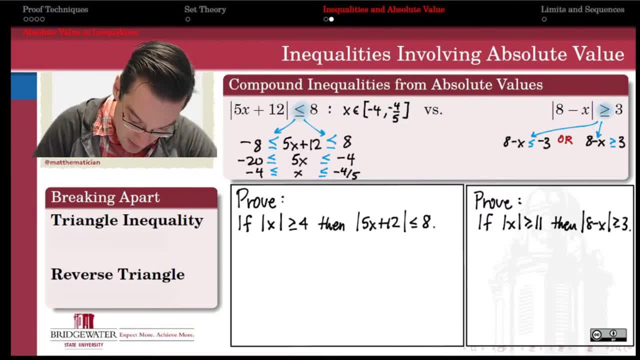 and which is a subtle difference, but it's an important one- logically, and then we would just solve each one of these inequalities in its own right, subtracting 8 from both sides, which does not reverse the inequality- minus X is less than or equal to negative 3 minus 8 is negative 11, and then multiplying both. 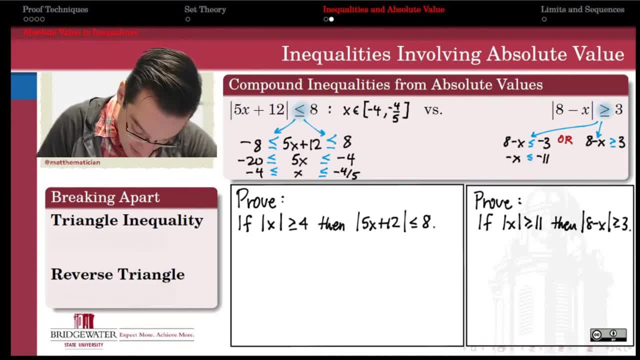 sides by negative 1, which is a decreasing operation. f of X equals minus X is a decreasing function, and so I do need my inequality to flip when I apply that last step- X greater than or equal to 11. do the same process for the other inequality: subtracting 8, it's going to give me a negative 5. 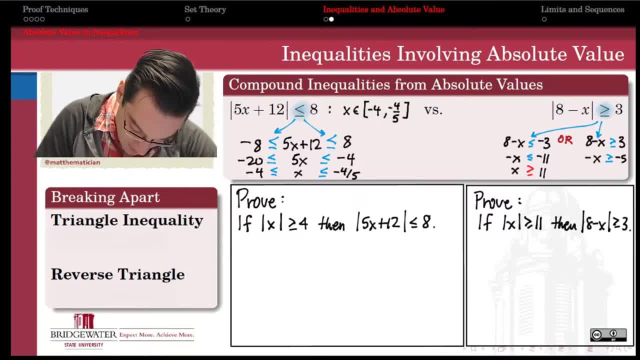 over here, minus X is greater than or equal to minus 5, and then again, when I multiply both sides by negative 1, that is a decreasing operation- the sense of my inequality reverses: X less than or equal to 5, and so the solution set of 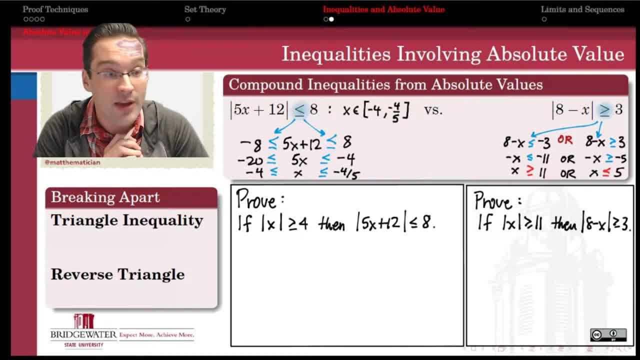 this inequality is all the X is greater than or equal to 11, together with all the X's that are less than or equal to 5, and so, as a union of two intervals, that would be the interval from minus infinity to 5, inclusive of 5, and the interval from 11 to positive infinity, inclusive of 11. 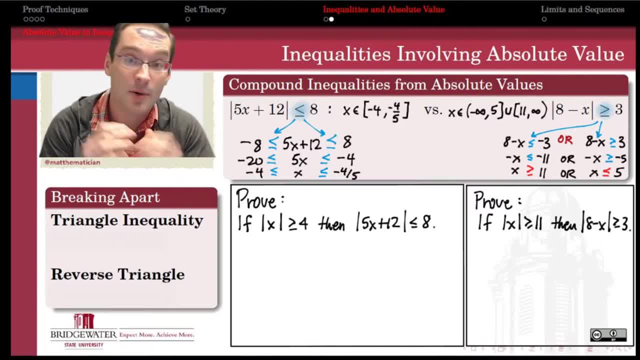 union together, and so the solution set for that inequality has these two unbounded pieces of the real line, going from 11 up to positive infinity and going from 5 down to negative infinity. so that's how we solve absolute value inequality, but that's, again, often not what we end up doing in real analysis in. 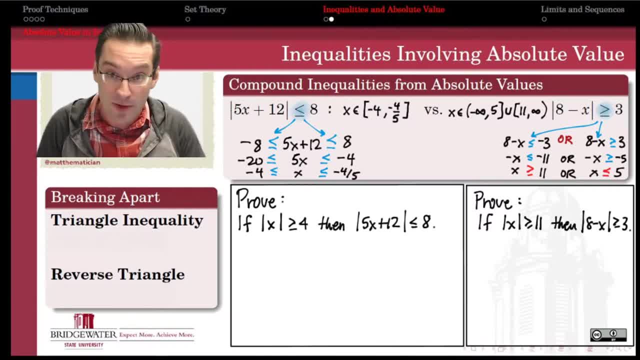 real analysis. we often have to substantiate absolute value inequalities as part of a proof, so they might look something more like what we have written down here, kind of one of these if-then statement. let's suppose we want to prove that if X is greater than or equal to 4 in absolute value, then we are guaranteed that the 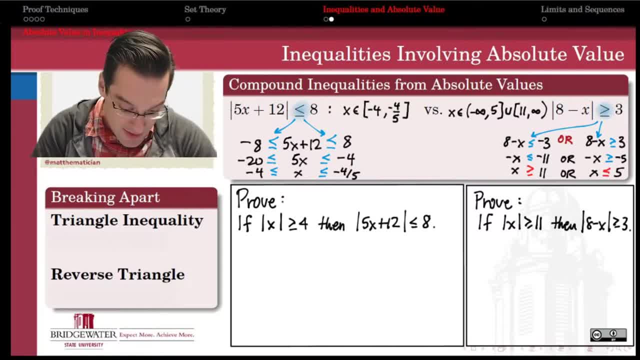 absolute value of 5x plus 12 is less than or equal to 8, and so if we didn't know any better, what we would probably do is just solve the inequality the way that we did up here and then try to draw the conclusion: oh, if the X is greater, 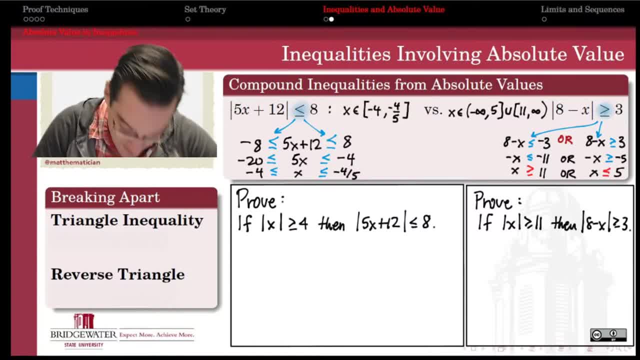 than or equal to 4 in absolute value. sorry, that inequality symbol is going the wrong way. typo- not my first typo today. we do need to fix it less than or equal to 4 and we would just say: well, if absolute value of X is less than or equal to 4, then we know that in. 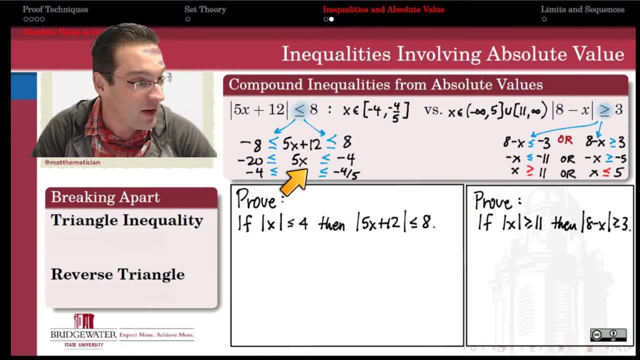 particular, it would be you know a part of this interval and we'd be able to make this conclusion, but what it looks like in real analysis is often different. so when we try to do a proof of this, what we start with if we're going to do, 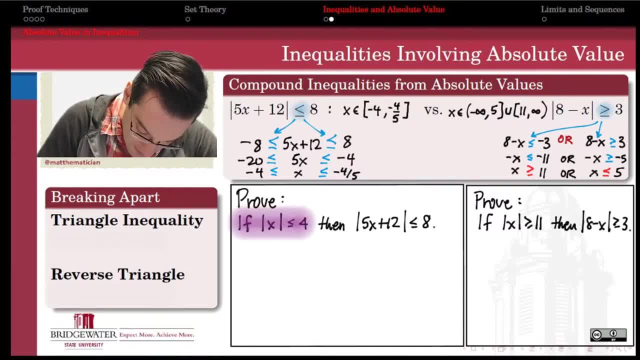 a direct proof, right is. we'll start with the statement where we stipulate: assume that the absolute value of X is less than or equal to 4, and so now what we want to do is to try to justify why the absolute value of 5x plus 12 is less. 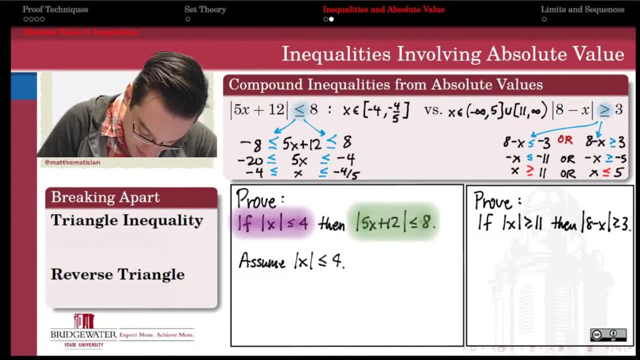 than or equal to 8, and so, like good students of proving inequalities, we would start with that left hand side, the way that we talked about on our first video today. I would start with the absolute value of 5x plus 12, and I want to try to take a bunch of steps. 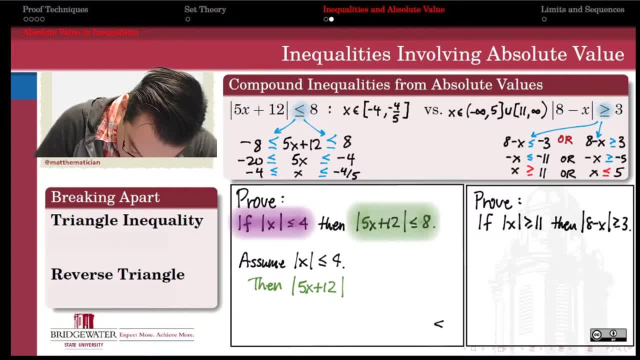 that show that I can get that quantity to be less than or equal to 8.. The problem is that I don't know anything about the absolute value of 5x plus 12, but I do know something about the absolute value of x, right, because that was my assumption here. So what I need is a tool. 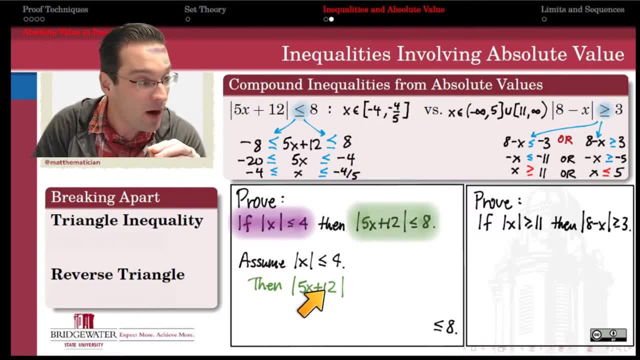 that can let me go inside those absolute value signs and break apart the absolute value over this plus that I have here in the middle. right, I don't want that plus. If I can get something like the absolute value of 5x by itself, we can work with that. 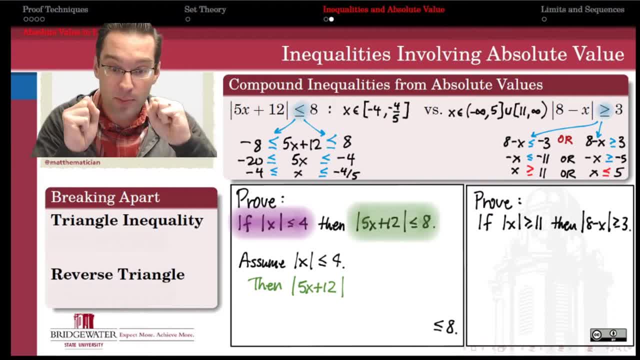 but 5x plus 12 we can't do anything with. So we want something that can break apart a plus or minus inside an absolute value, and that is what the triangle inequality does for us. The triangle inequality tells me that for any real numbers, x and y, the absolute value of a sum. 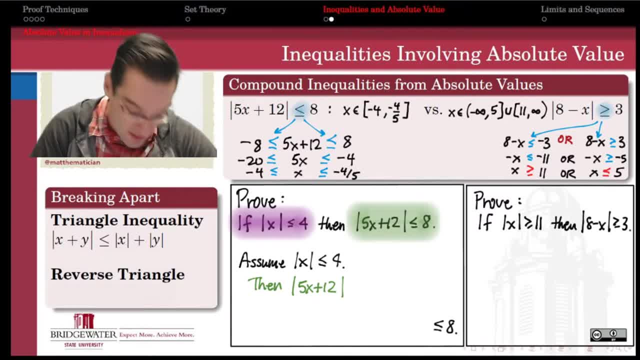 is less than or equal to the sum of the absolute values. Again, this is probably the a number one most important tool in your real analysis toolbox. You're going to write a lot of proofs using the triangle inequality at some point during the semester, So let's see if this triangle inequality can help us. 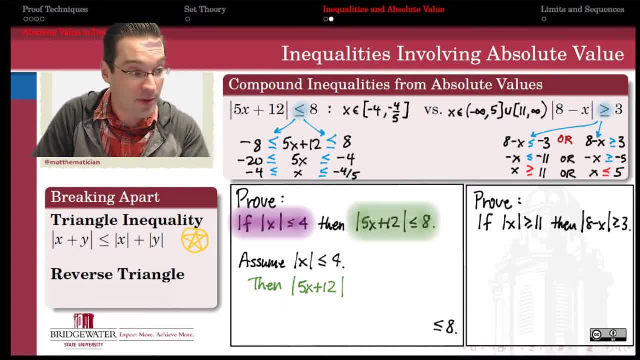 If I were to apply it to the absolute value of 5x plus 12, what it would tell me is that the absolute value of 5x plus 12 is less than or equal to- And that's good, by the way, right, because I'm trying to replace this with: 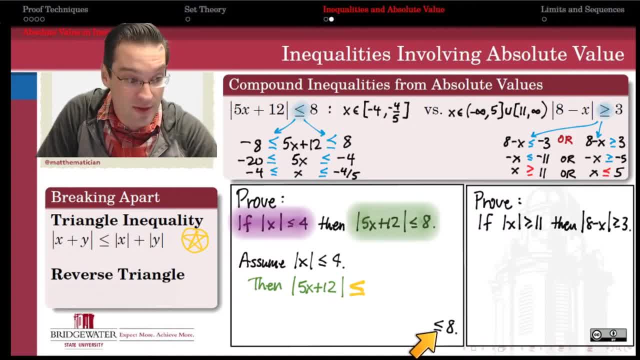 something bigger, with something bigger, with something bigger, because ultimately, I need to show that it's less than or equal to something. So this inequality is going in the right direction for what we want. And now, applying the triangle inequality, we'll know that that's less than or equal to the absolute value of 5x. 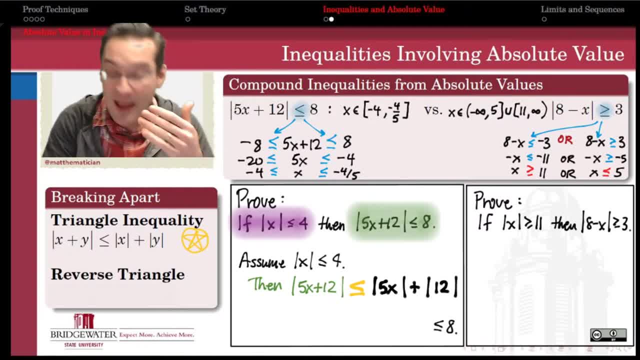 plus the absolute value of 12.. And that's super good now, because I have my x in its own term, with its own absolute value right now, which will be helpful because we should ultimately be able to apply this assumption to it. Well, the absolute value of 12. 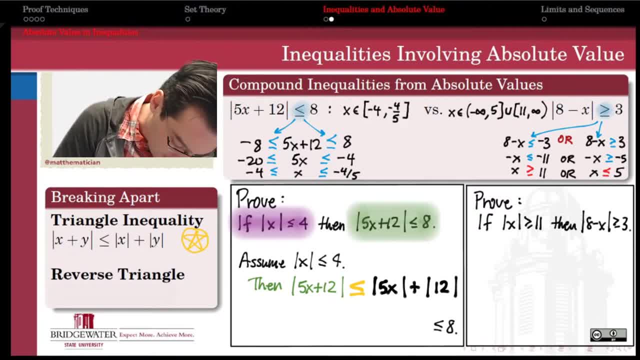 is just 12, so we don't have to worry about that term on the end having any sort of weirdness. I'm just going to put an equal sign here for a minute. Absolute value of that 12 is equal to 12.. What about the absolute value of 5x? Well, one of the properties that absolute 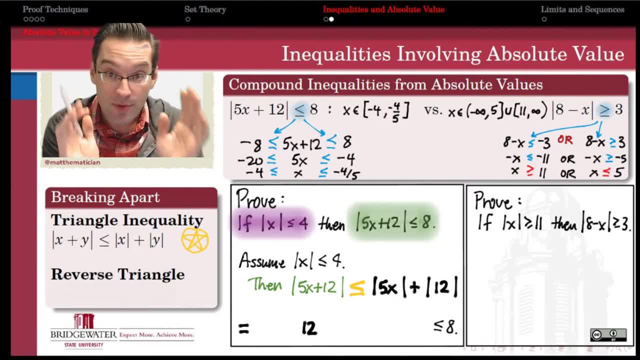 values have in real numbers is that they are multiplicative. The absolute value of a product is exactly equal to the product of the absolute values. So the absolute value of 5x is equal to the absolute value of 5 times the absolute value of x. right, But the absolute value of 5 is just 5, because 5 is 5 units away. 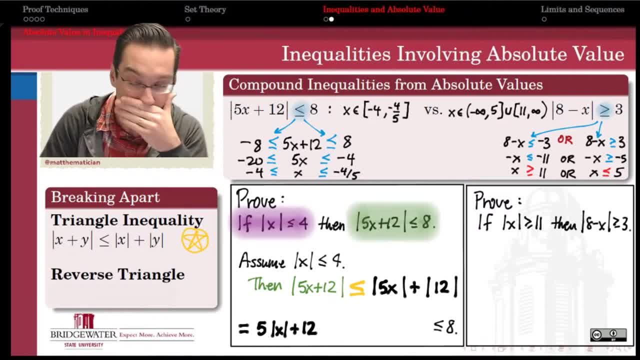 from 0 on the number line. And so now that I have the absolute value of x by itself, now we have our magical assumption, I can use my assumption by my assumption that absolute value of x is less than or equal to 4.. Now I see that I've got maybe a problem with this. 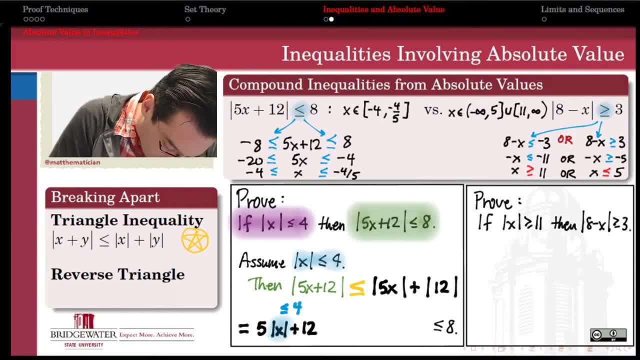 But let's forge ahead. for the moment, This is less than, or equal to 4.. And so, therefore, this is less than, or equal to whoops. I'll try and keep my color coding: less than, or equal to, 5 times 4 plus 12.. 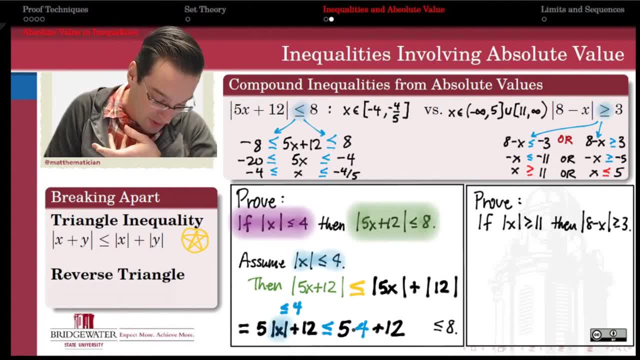 And I've got a problem right, because 5 times 4 plus 12 is not in fact less than or equal to 8. So I screwed something up here, And you might be able to tell why it is that this didn't work. 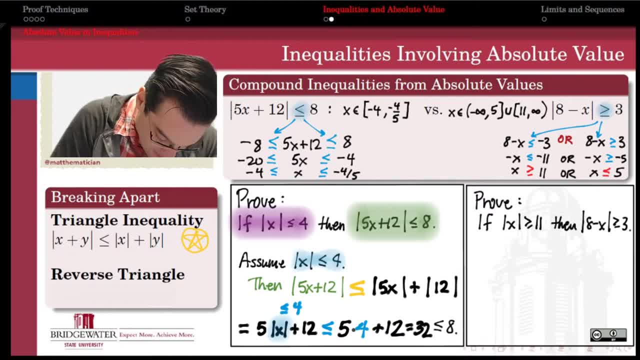 So maybe you can tell why this didn't work: because there are values of x that are less than 4 in absolute value that don't actually belong to this solution set that we discovered up here. So yeah, so I messed that up. What I meant to put. I think what I meant to put here was negative 4, was 4 fifths rather. 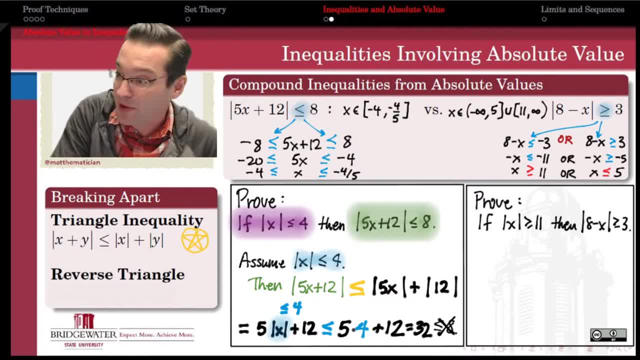 than 4.. So let's rewind the tape real quickly and I'm just going to make that correction So we'll see how this proof was actually supposed to have worked. So yeah, my apologies on this one. I had written the statement of this problem incorrectly. 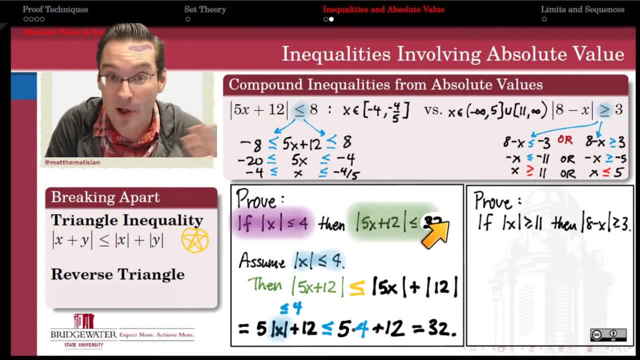 What we wanted was 32 here and not 8.. So of course you all can't change the problems when you're solving them in analysis. But you know, as an instructor writing a problem, I wrote one that didn't work, So let's change it to one that did. 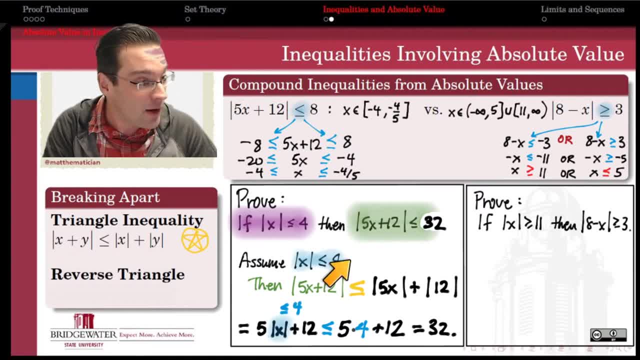 The important part is the structure of the proof. right, We started out with absolute value of 5x plus 12,, which we didn't know anything about. But we made an assumption about the absolute value of x And our tool for turning the expression absolute value of 5x plus 12,, which is unknown, into. 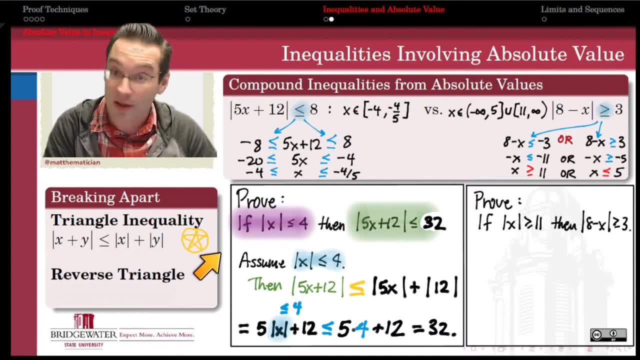 an expression that involves the absolute value of x plus 12, which is unknown- into an expression that involves the absolute value of x, which we do know is the triangle inequality. It lets us break apart an absolute value over a sum. The absolute value of a sum is less than or equal to the sum of the absolute values. 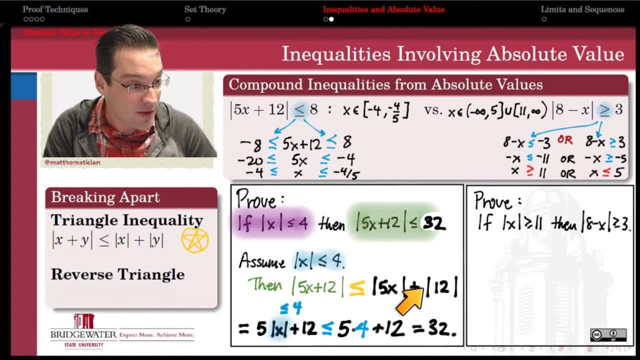 And now reading this from left to right: absolute value of 5x plus 12 is less than or equal to less than or equal to 32.. Which is, you know what I should have written as the original problem. So what's different if we don't want a less than or equal to here, but we want a greater? 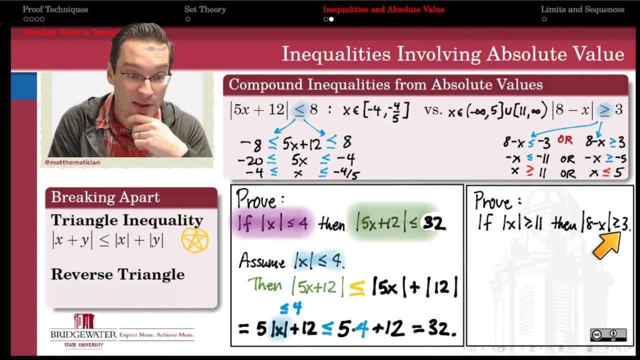 than or equal to. Let's suppose I'm trying to establish that value of 8 minus x is greater than or equal to 3, if I know that the absolute value of x is greater than 11, right, We need a different kind of triangle inequality called the reverse. 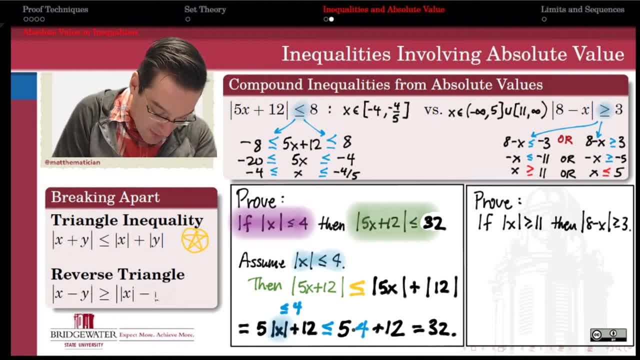 triangle inequality And the reverse triangle inequality tells us something about the absolute value of a difference- x minus y- rather than the absolute value of a sum. It says that the absolute value of the difference of x and y is greater than or equal to the difference. 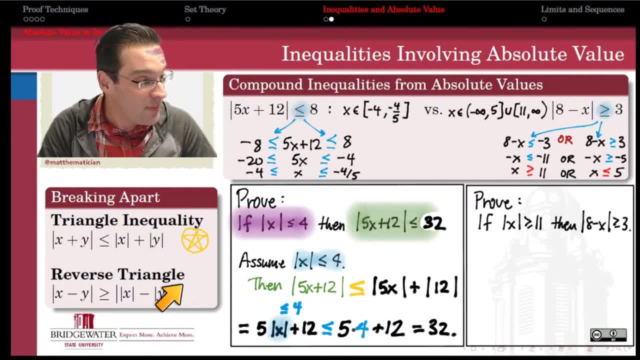 between the absolute values of x and the absolute values of y, but with an extra set of absolute value symbols on the outside of it, because we don't necessarily, if absolute value of x minus absolute value of y is negative, we want to flip that so that it's positive. so 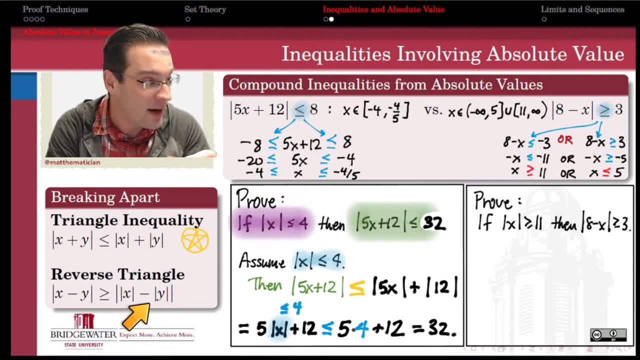 that we're saying something interesting. Otherwise, we could end up with this thing on the right hand side being negative and of course we know the absolute value of something is going to be greater than or equal to a negative quantity. So, to make it say something more profound, we have this extra set of absolute values. 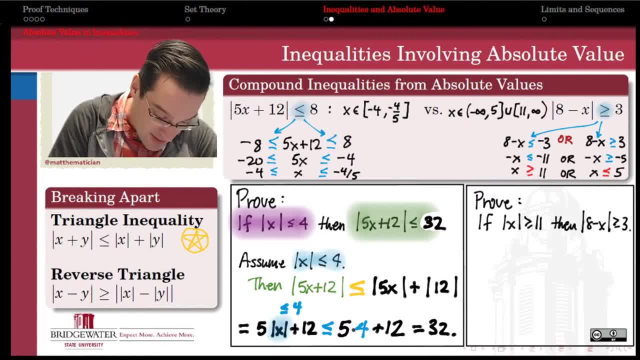 on the outside. This is the reverse triangle- inequality. So let's use that to prove this last example, which definitely does work, that if the absolute value of x is greater than or equal to 11, so that's going to be the thing that we stipulate. 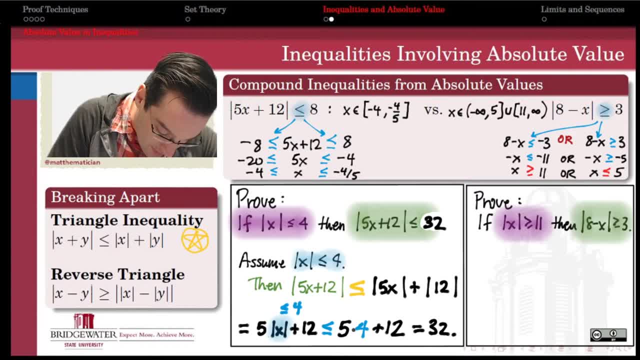 that's going to be what we assume to be true, and we want to try to prove that absolute value of 8 minus x is greater than or equal to 3.. So we'll start by making the assumption- Assume that we know that the absolute value of x is greater than or equal to 11- and now 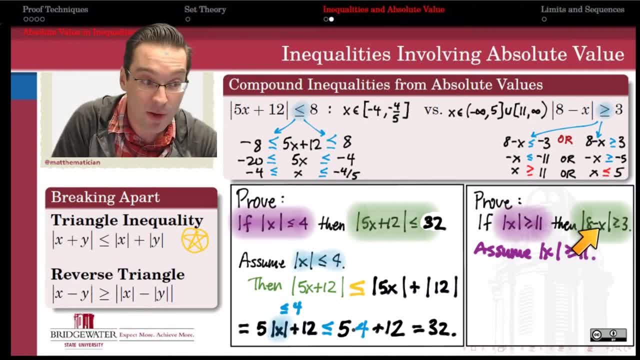 dutifully. we will try to work from the left side of this inequality which we're trying to prove and make it arrive at the right hand side. So the absolute value of 8 minus x. We want to show that somehow this is greater than or equal to 3, so we have to get from. 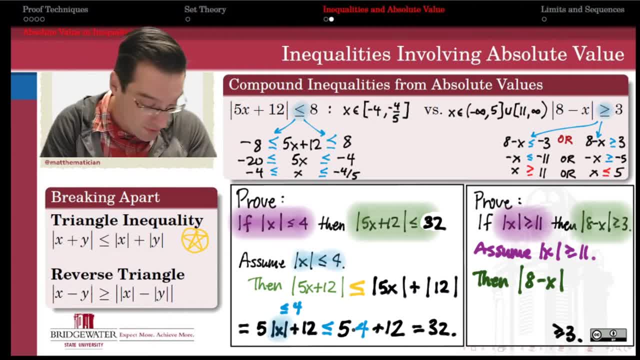 here to there. How do we do it? Let's apply the reverse triangle inequality, which we would do because we have a subtraction in here. so that's one clue, but the more important clue is that we're trying to bound this absolute value from below. 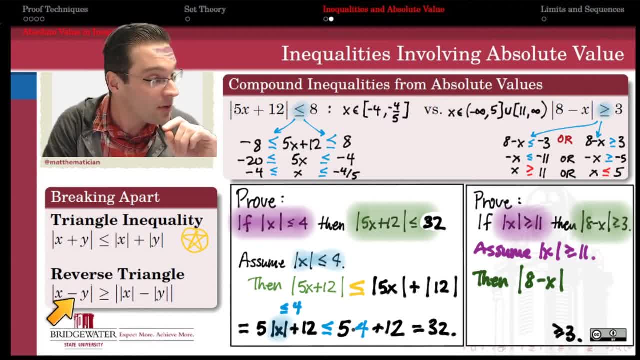 We want a greater than or equal to here, and not a less than or equal to, And so the reverse triangle, inequality that has the greater than or equal to on this side of the absolute value, is the one that we know that we should use. So the absolute value of 8 minus x is greater than or equal to 11.. 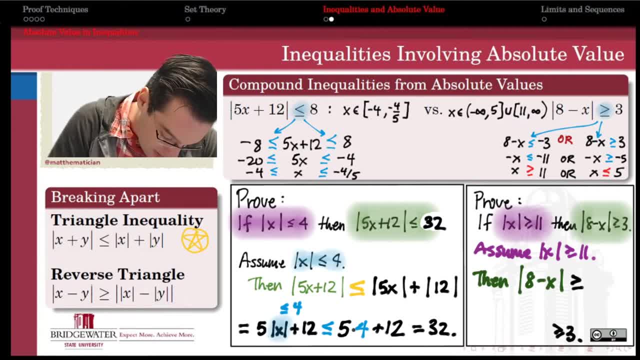 So we want to show that somehow this is greater than or equal to 3, so we have to get from here to there. So the absolute value of 8 minus x is greater than or equal to. according to the reverse triangle inequality, this one is going to be greater than or equal to the absolute value. 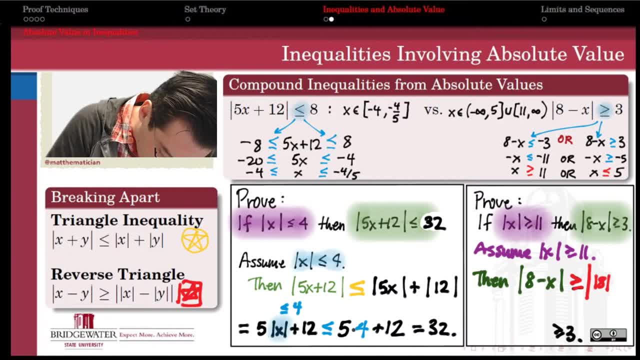 of the absolute value of 8 minus the absolute value of x. So you're going to end up with a lot of vertical lines and it's going to look a little bit confusing at first. But let's simplify it just a little bit. The absolute value of 8 is just 8, and so we can just write 8 minus the absolute value. 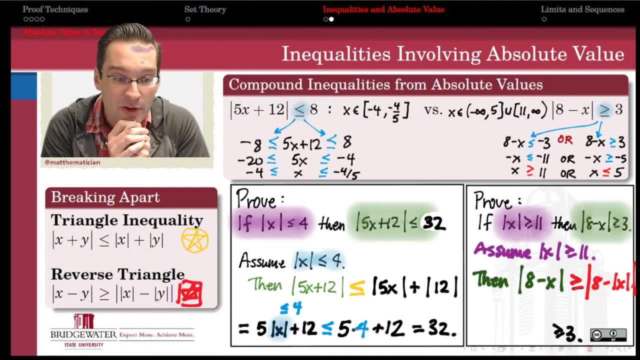 of x. But now we want to do a little bit more thinking right, because we have this big set of absolute value bars on the outside that we want to try to do something with. Let's go back to our assumption. We know the absolute value of x is at least 11.. 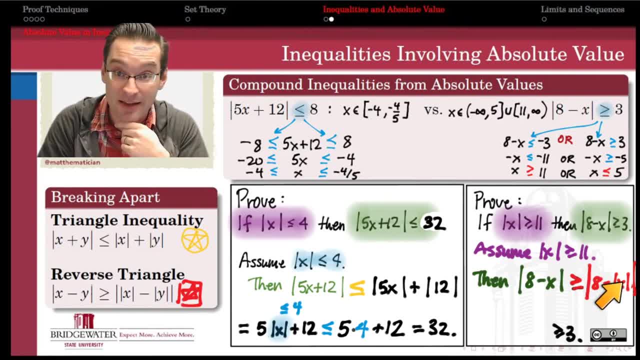 So if I take 8 and subtract a number which is at least 11, we know for sure that 8 minus something which is bigger than 11 is going to be a negative real number, And so the absolute value of a negative quantity is the opposite of that quantity. 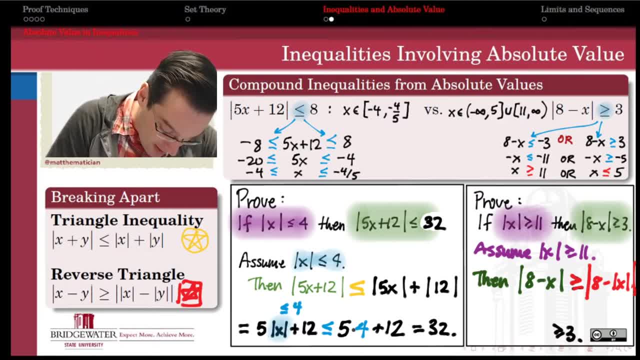 So the absolute value of 8 minus the absolute value of x is going to be equal to the opposite of 8 minus the absolute value of x, because 8 minus that thing is negative, And so the absolute value of 8 minus that thing is going to be the opposite, the positive. 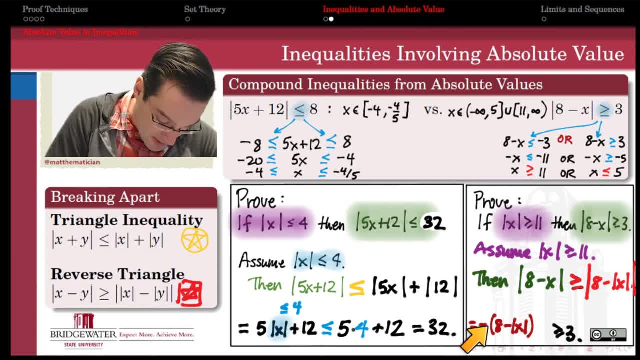 version of 8 minus the absolute value of x, And so when I distribute this minus sign, I'm going to get absolute value of x minus 8 instead of 8 minus the absolute value of x. And now we have the absolute value of x right where we want it, because we happen. 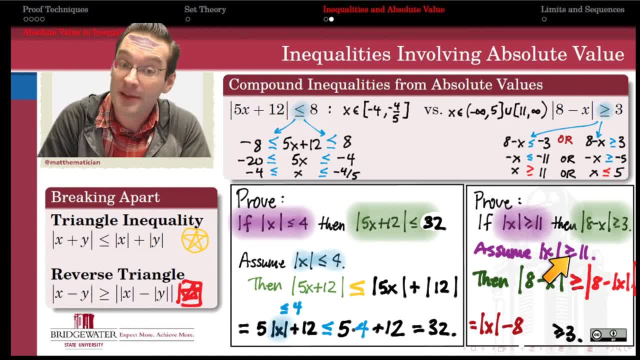 to know something about the absolute value of x. We assumed that it was greater than or equal to 11.. And so now we can apply that assumption. This absolute value of x is greater than or equal to 11, and therefore absolute value of x minus 8 is greater than or equal to 11 minus 8.. 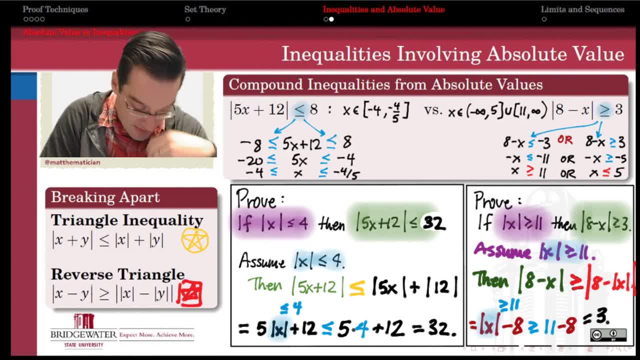 And 11 minus 8 just happens to be 3.. And if I read this inequality from left to right, we've proven exactly what we set out to prove. The absolute value of 8 minus x is greater than or equal to, and at every step we replaced: 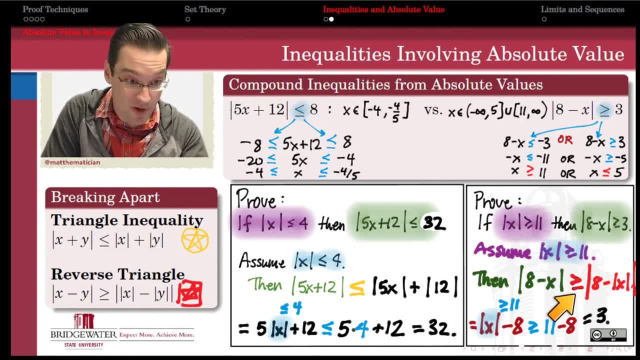 this with either something which was less than or equal to it, or something which is equal to it. So all my inequality symbols are going in the same direction, which is always what we need when we're solving an inequality. Absolute value of 8 minus x is greater than or equal to 11 minus 8.. 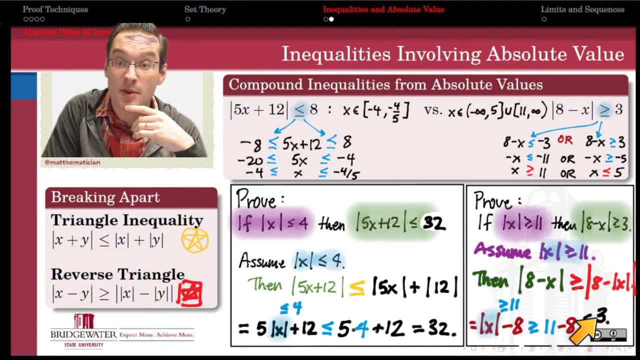 Greater than or equal to something which is equal to something which is greater than or equal to something which turns out to be 3.. And that completes the proof. So these are just the extra steps that you have to do when the absolute value comes to. 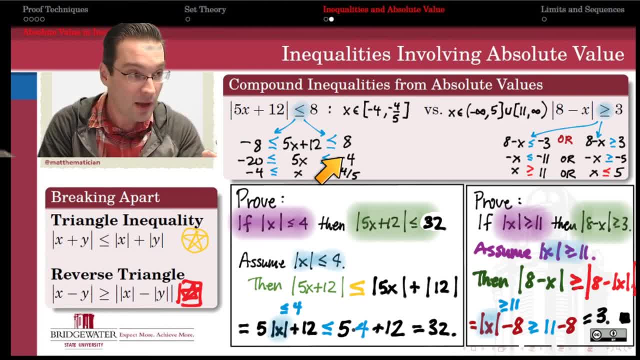 the party Is that if you're solving an inequality, break it apart into a compound inequality and solve each of those pieces individually. But more frequently, in real analysis, when you're using an absolute value- inequality in a proof- the triangle inequality and its alter ego, the reverse triangle inequality. 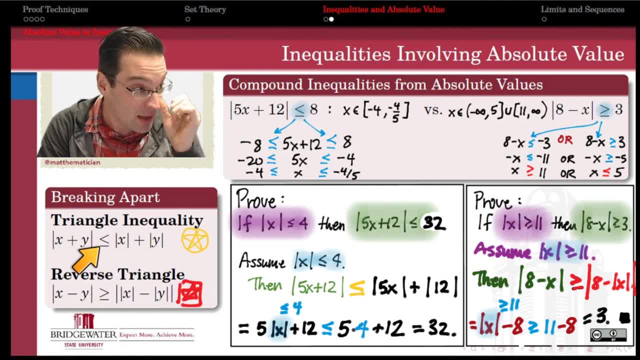 are your friends Any time you're trying to establish an inequality that has an absolute value bounded from above. so less than or equal to, right here the triangle inequality, the original one is your tool. So that's what we did here, right? absolute value of 5x minus 12 is less than or equal.